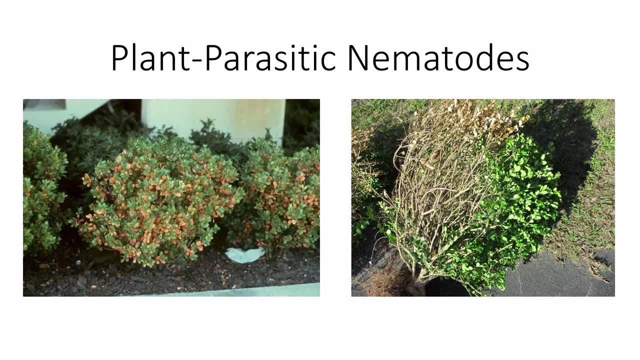 damage caused by them is so subtle that it goes unnoticed or is attributed to other causes. In this video, I will discuss the types of nematodes and how to diagnose nematode problems. Some scientists estimate that there are over 1 million kinds of nematodes making them. 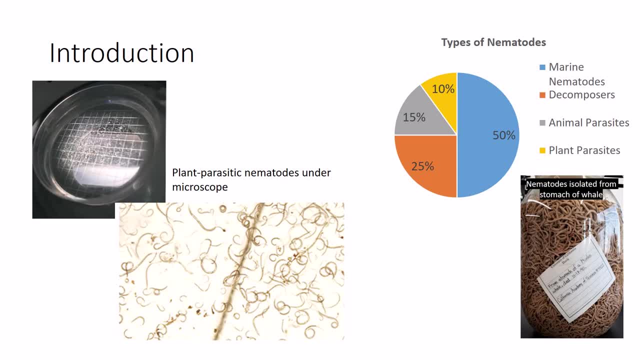 second only to the insects in numbers. However, few people are aware of nematodes or have seen any, because nematodes are very small, even are microscopic and colorless. Most live hidden in soil, underwater or in the plants or animals they parasitize And relatively 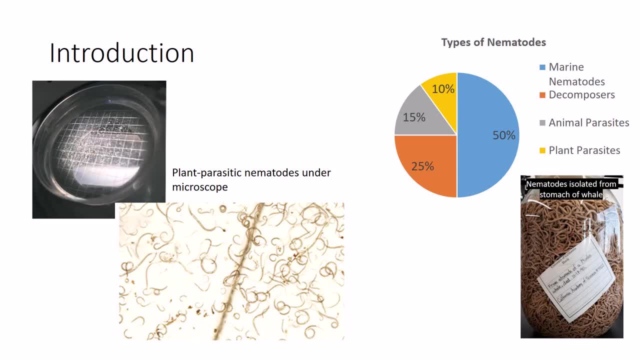 few have obvious direct effects on humans or their activities. Of all the nematodes known, about 50% live in marine areas. Some nematodes are known for their presence in the soil, underwater or in the plants or animals they parasitize, and relatively few have obvious direct effects on humans or their activities. Of all the nematodes known, about 50% live in marine. 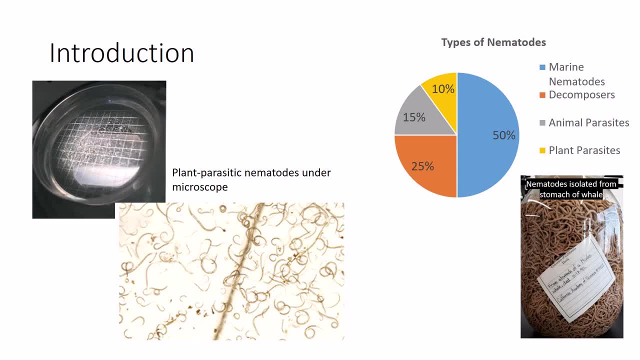 environments and 25% live in the soil or freshwater and feed on bacteria, fungi, other decomposer organisms, small invertebrates or organic matter. About 15% are parasites of animals, ranging from small insects and other invertebrates up to domestic and wild. 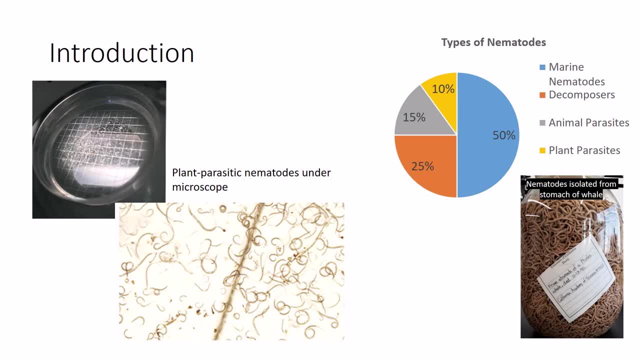 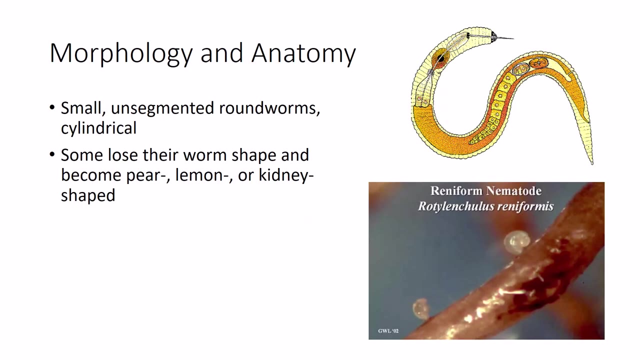 animals and man. Some of the parasites of animals are the largest nematodes known. Some from grasshoppers can be several inches long and one from whales can reach lengths of more than 20 feet. Only about 10% of known nematodes are parasites of plants. 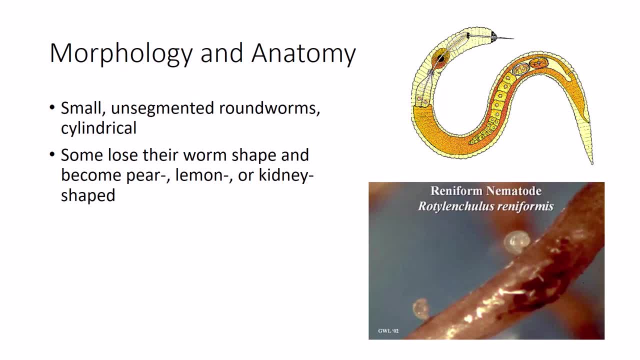 Plant nematodes are tiny, unsegmented roundworms that are cylindrical, tapering toward the head and tail. Females of a few species lose their worm shape as they mature, becoming pear, lemon or kidney shaped. Plant parasitic nematodes possess all of the major organ systems. 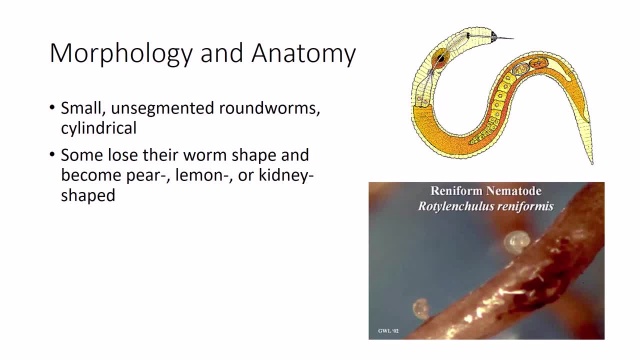 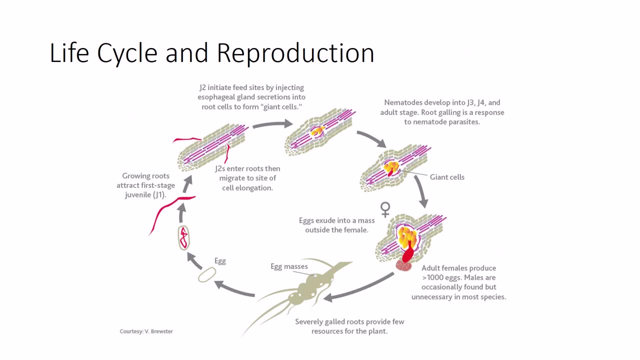 of higher animals, except respiratory and circulatory systems. The body is covered by a transparent cuticle which bears surface marks helpful for identifying nematode species. The life cycle of a plant. parasitic nematode has six stages: egg, four juvenile stages and adult. Male and female nematodes occur in most. 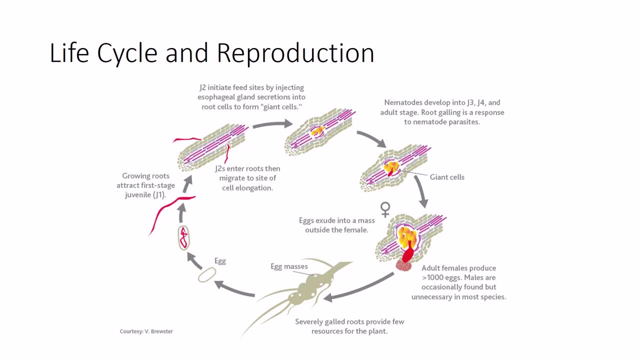 species, but reproduction without males is common and some species are hermaphroditic. Females produce both sperm and eggs. Egg production by the individual completes the life cycle. Most species produce between 50 and 500 eggs per female, depending on the nematode species. 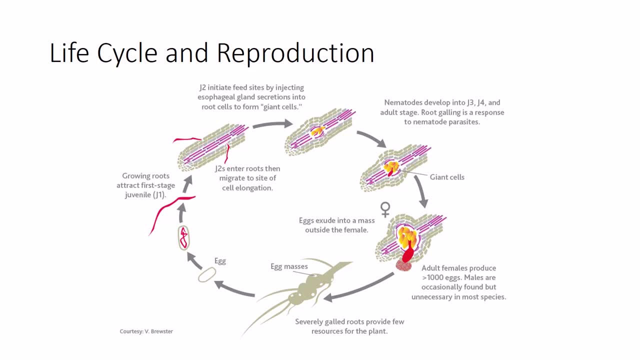 and their environment, but some can produce more than a thousand eggs. The length of the life cycle varies considerably depending on nematode species, host plant and the temperature of the habitat. During summer months, when soil temperatures are 80 to 90 degrees Fahrenheit, many plant nematodes 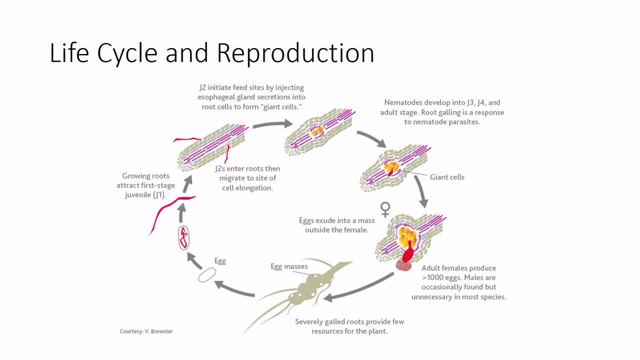 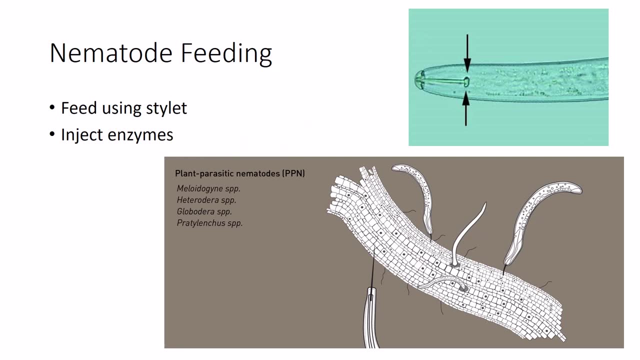 complete their life cycle in about four weeks. On the slide you can see the life cycle of a plant parasitic nematode. Plant parasitic nematodes feed on living plant tissues using an oral stylet, a spearing device, somewhat like a hypodermic needle, to puncture host cells. Many, probably all, 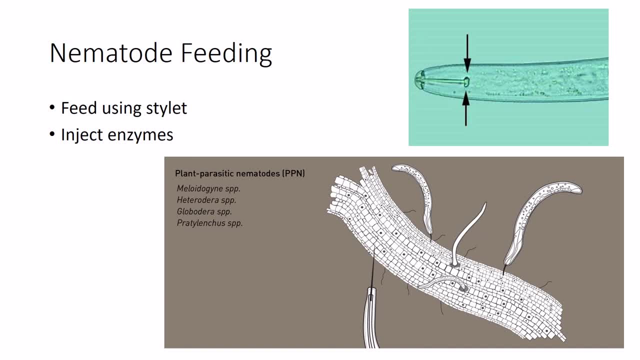 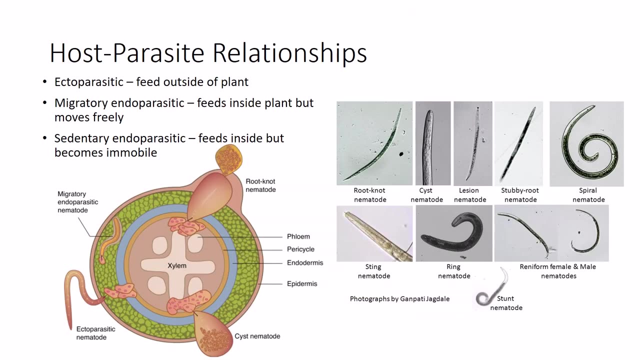 plant nematodes inject enzymes into a host cell before feeding to partially digest the cell contents before they are sucked into the gut. Most of the injury that nematodes cause plants is related in some way to the feeding process. Ectoparasitic nematodes feed on plant tissues from outside the plant. Endoparasitic nematodes: 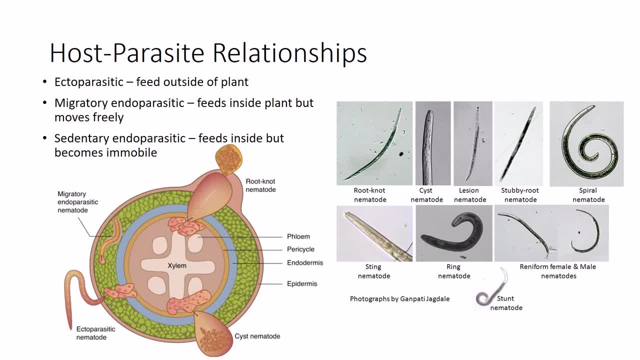 feed inside the tissues. If the adult female moves freely through the soil or plant tissues, the species is said to be migratory. Species in which the adult females become swollen and permanently immobile in one place, in or on a root, are termed sedentary Migratory endoparasitic. 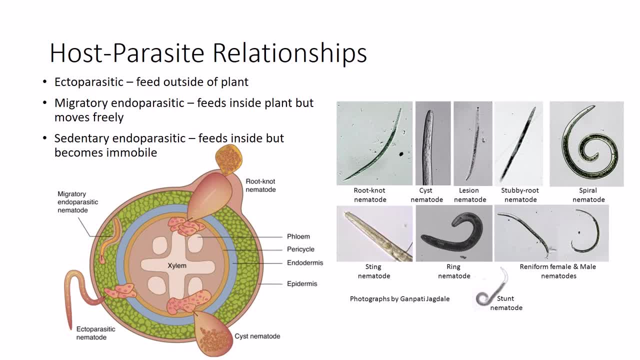 and ectoparasitic nematodes feed on plant tissues from outside the plant. Endoparasitic nematodes generally deposit their eggs singly, as they are produced wherever the female happens to be in the soil or plant. Sedentary nematodes such as root knot, cyst, reniform and citrus nematodes produce. 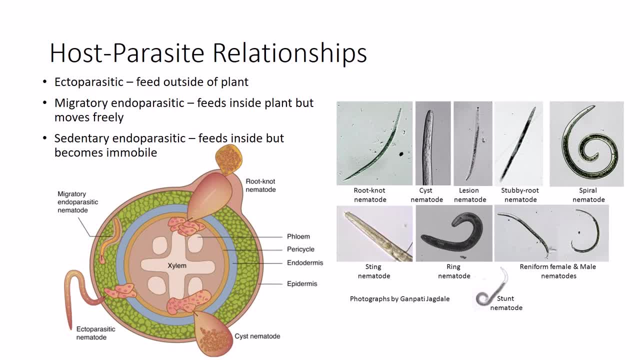 large numbers of eggs which remain in their bodies or accumulate in masses attached to their bodies. The feeding-slash-living relationships that nematodes have with their hosts affect sampling methods and the success of management practices. Ectoparasitic nematodes, which never 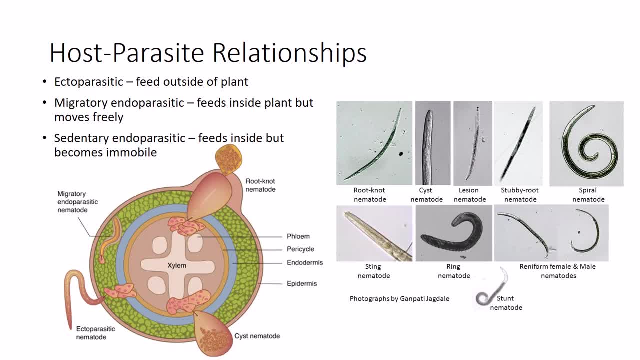 enter roots May be recovered only from soil samples: Endoparasitic nematodes, which are often detected most easily in samples of the tissues in which they feed and live, Burrowing and lesion nematodes, But some occur more commonly as migratory stages in the soil, Root knot and 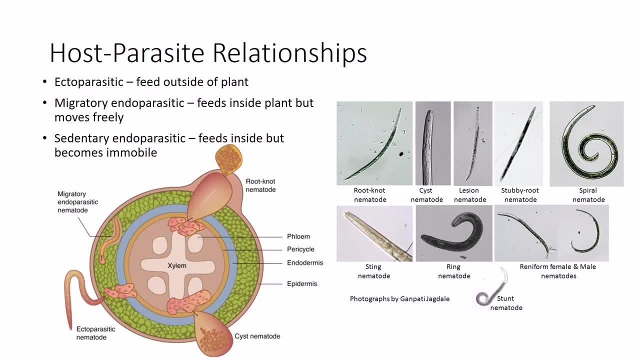 reniform nematodes. Endoparasitic nematodes inside root tissues may be protected from those kinds of pesticides that do not penetrate into roots. Root tissues may also shield them from many microorganisms. Endoparasitic nematodes may be recovered only from soil samples. Endoparasitic 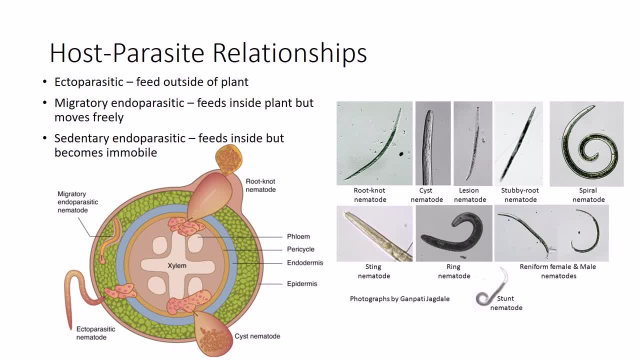 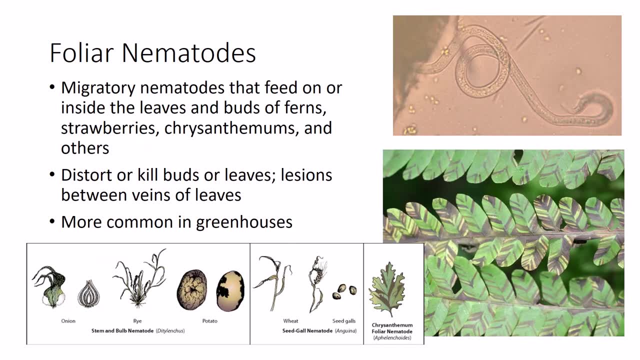 nematodes can attack nematodes in the soil. Ectoparasites are more exposed to pesticides and natural control agents in the soil. Foliar nematodes are migratory nematodes that feed on or inside the leaves and buds of ferns, strawberries, chrysanthemums. 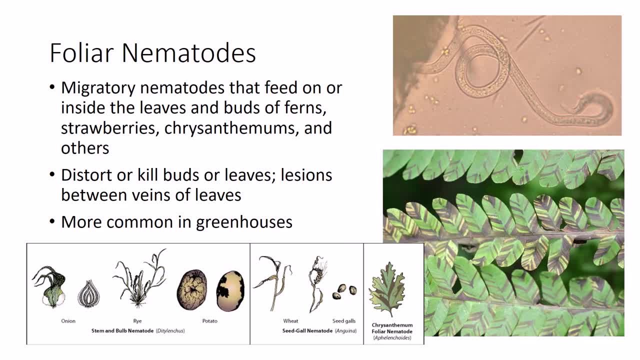 and many other ornamentals. These are more common in greenhouses where the humidity is high. They cause distortion and death of buds, leaf distortion or yellowing of the leaves. The nematodes are more exposed to pesticides and natural control agents in the soil. 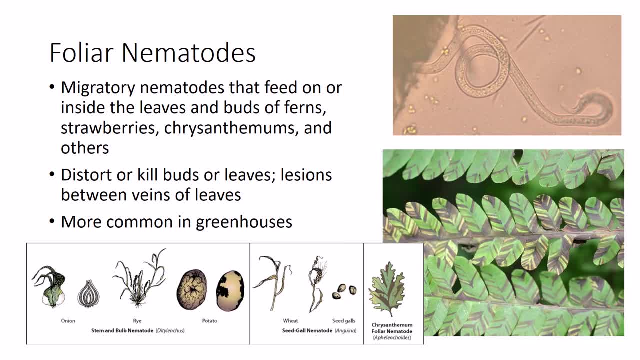 Ectoparasites are more exposed to pesticides and natural control agents in the soil, or yellow to dark brown lesions between major veins of leaves. Their symptoms may be mistaken for bacterial infections. Other nematodes that attack plants above ground but are not common. 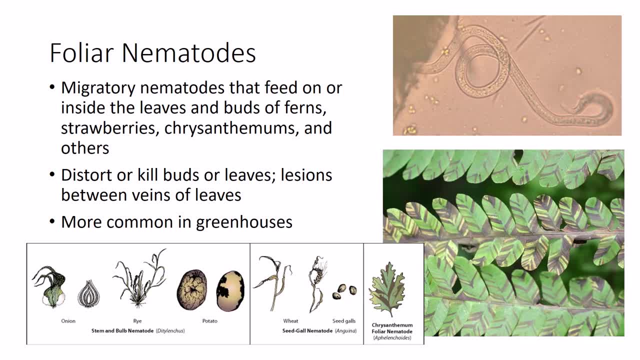 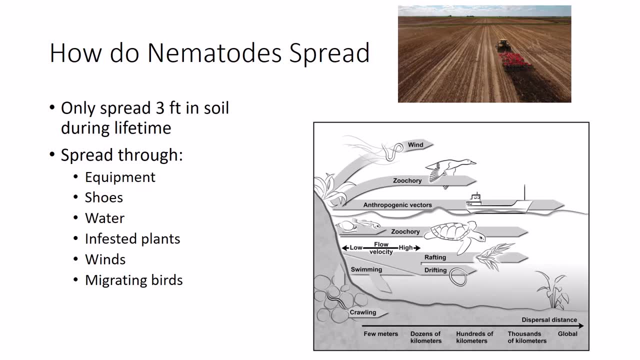 in Florida, cause leaf or seed galls. Still others cause deterioration of the bulbs and necks of onions and their relatives. While nematodes are mobile animals, most are able to move no more than three feet through the soil within their lifetime. However, this lack of long-distance 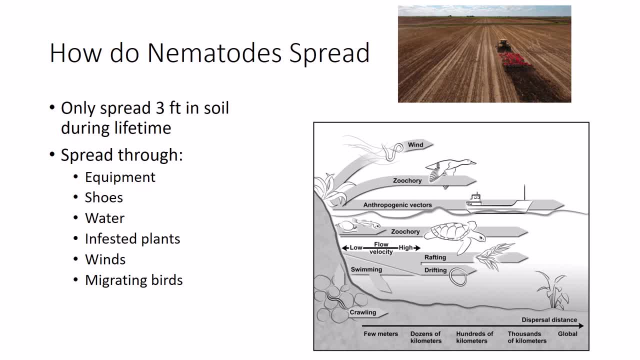 crawling does not mean nematodes cannot rapidly spread from field to field. Farm equipment and even muddy shoes contaminated with nematode-infested soil can rapidly disperse nematodes. The movement of water during floods and irrigation can disperse nematodes over long distances. 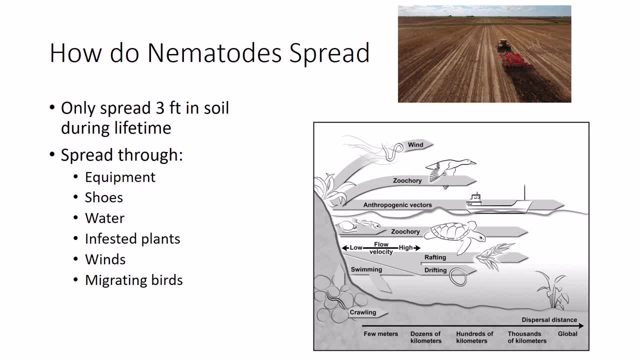 Likewise, the movement of nematode-infected plants, seeds and bulbs can give nematodes international tickets to travel the world, if plant quarantine officials are not. The ability of nematodes to form environmentally resistant stages make their dissemination even easier, since dried nematodes can be blown with the wind or plant debris over large 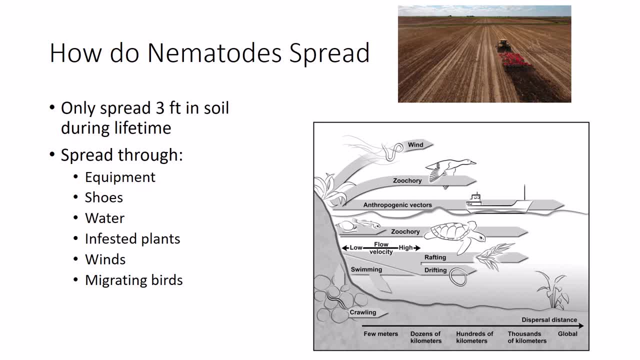 geographical regions. Even migrating birds are suspected to be able to carry nematodes along their flight paths, assisting the nematodes in their quest for new homes. Essentially, any process that moves soil or plant tissue has the ability to disperse plant nematodes. 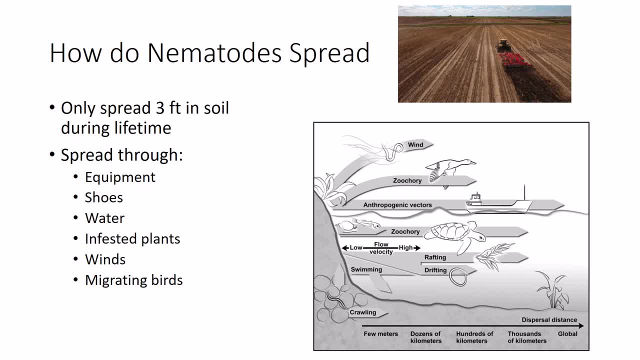 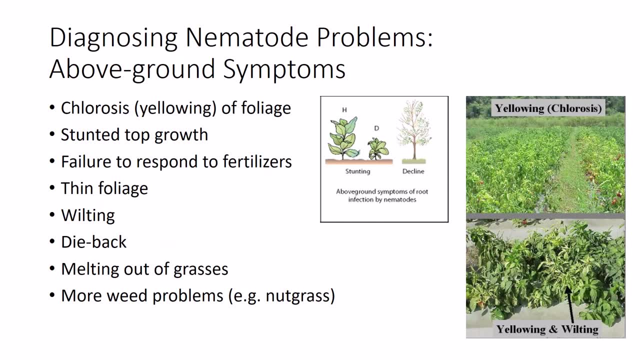 making them difficult. plant pathogens: Determining if nematodes are involved in a plant growth problem is difficult because few nematodes cause distinctive diagnostic symptoms. A sound diagnosis should be based on as many as possible of symptoms above and below ground, field history and laboratory. 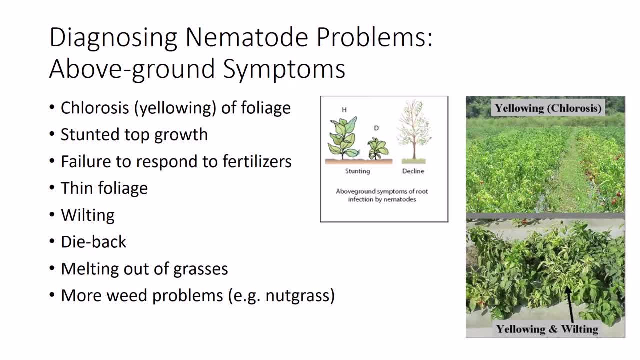 assay of soil and or plant samples. It is rare that above-ground symptoms give sufficient evidence to diagnose a nematode problem in the roots. However, they are important because they are almost always the reason that nematode problems are first noticed. Since most plant nematodes affect root functions, most symptoms associated with them are the result. 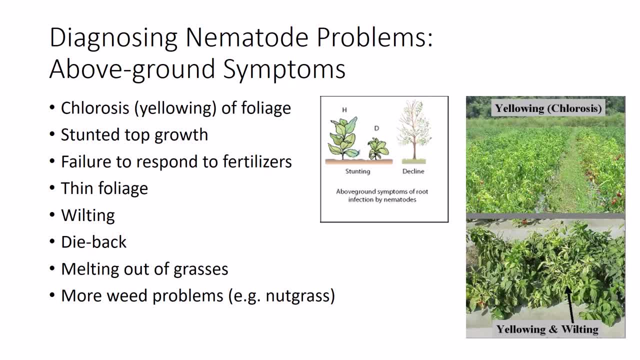 of inadequate water supply or mineral nutrition to the tops. chlorosis, yellowing or other abnormal coloration of the foliage. stunted top growth. failure to respond normally to fertilizers. small or sparse foliage. a tendency to wilt more readily than healthy plants. 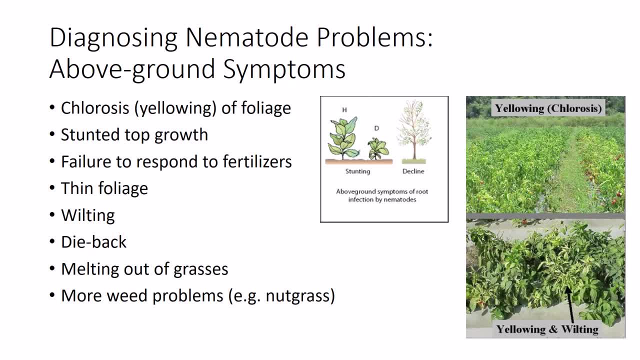 and slower growth. Over-recovery from wilting Woody plants in advanced stages of decline caused by nematodes may exhibit dieback of progressively larger branches. Melting out or gradual decline is typical of nematode-injured turf and pasture. Plantings stunted by nematodes often have worse weed problems than areas. 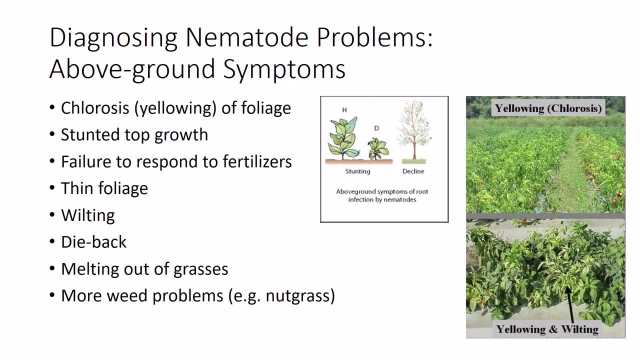 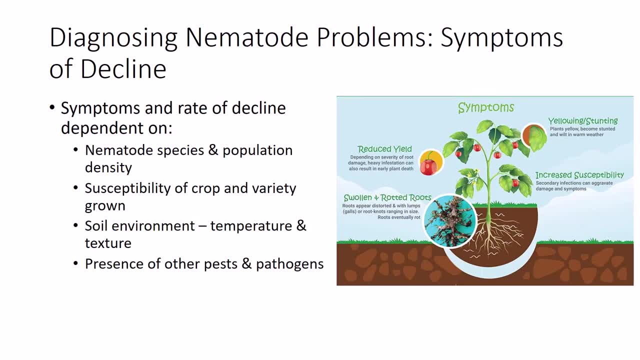 without them, because the crop is less able than it should be to compete with weeds. These symptoms can easily be mistaken for the effects of drought, general stress or fungus. The amount of symptoms and the rate of decline is dependent on several factors. First, some nematode. 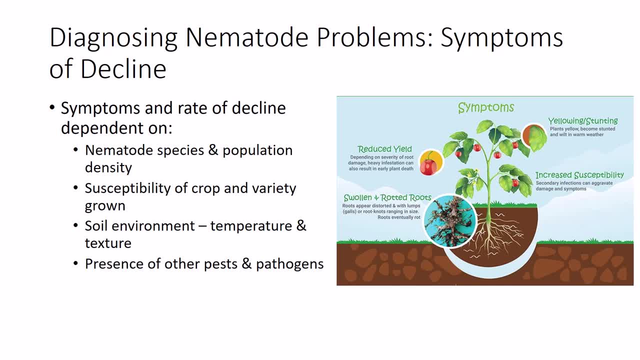 species cause more damage than others. In turfgrass, you only need 20 sting nematodes found in a sample to be considered damaging, while 100-ring nematodes are not even considered damaging at that amount. A greater population density of nematodes, especially the more damaging ones. 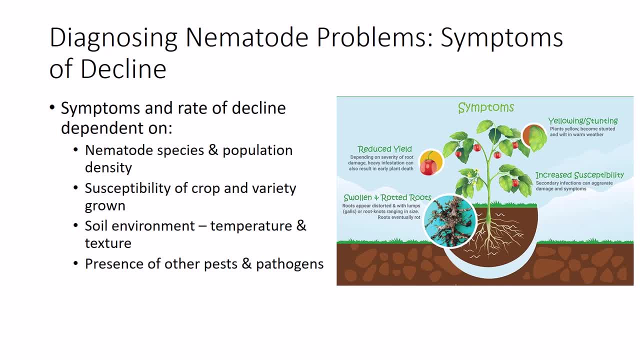 will cause greater symptoms. Additionally, some crops are more susceptible to nematodes than others. Some plants are very susceptible to nematodes and some plants are more susceptible to nematodes than others. Some varieties may be tolerant or resistant to nematodes. Nematodes are a greater problem. 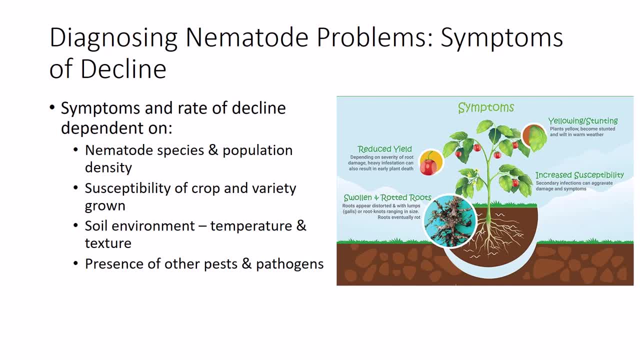 where conditions favor them, such as a long growing season, sandy soil and plants under water or nutrient stresses. Nematode feeding sites in the roots can also provide entrance for other disease-causing organisms like fungi or bacteria, leading to increased plant damage. 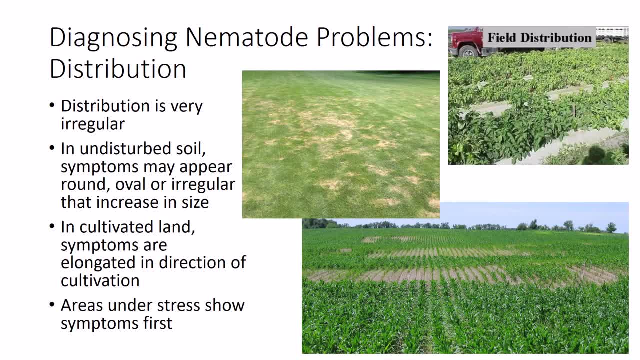 These are often called secondary infections. The distribution of nematodes within any site is very irregular, so the shape, size and distribution of areas with the most severe effects of nematodes will be erratic within the field. Nematodes move very few feet per year on their 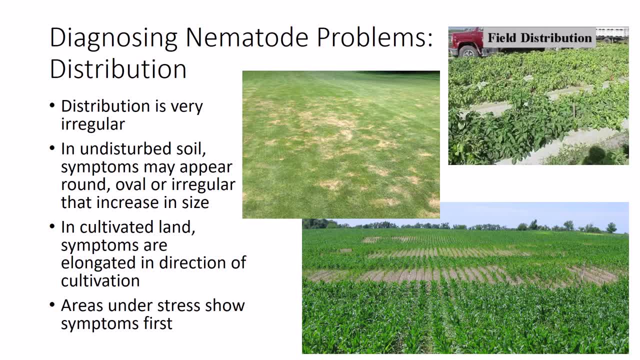 own In the undisturbed soil of groves, turf and pastures. visible symptoms of nematode injuries normally appear as round, oval or irregular areas that gradually increase in size year by year. In cultivated land, nematode injured spots are often elongated in the direction. 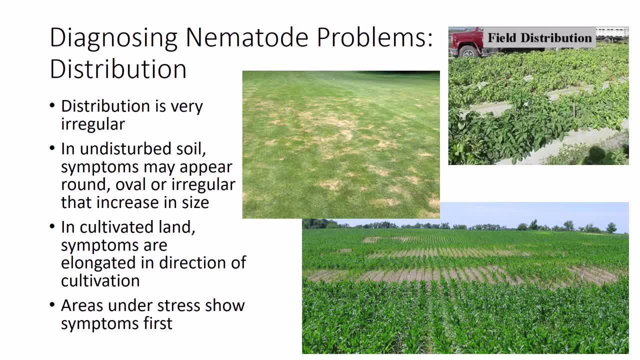 of cultivation In urban years. each year one nematode is going to have to governorally cultivation because nematodes are moved by machinery. Erosion, land leveling and any other force that moves masses of soil or plant parts can also spread a nematode infestation. 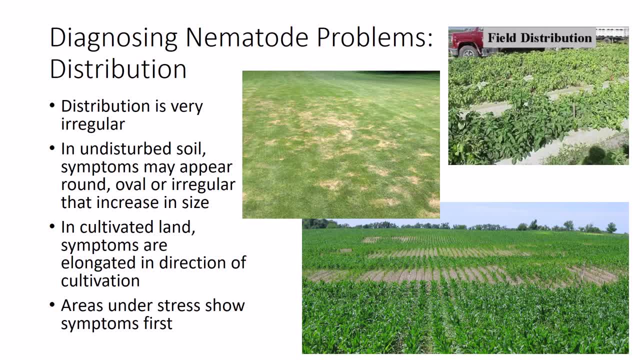 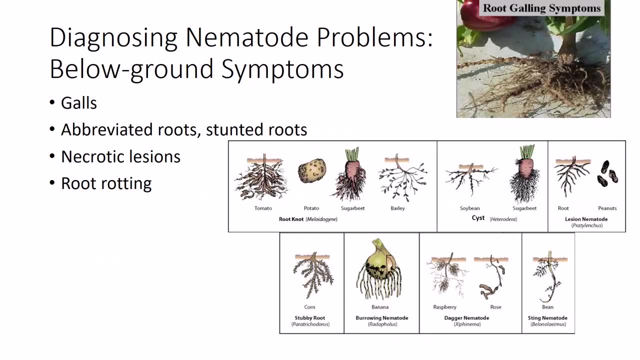 much more rapidly than it will go by itself. Nematode damage is often seen first and most pronounced in areas under special stresses such as heavy traffic, excessive drainage because of slope or soil and dry areas outside regular irrigation patterns. Below ground symptoms may be more useful than top symptoms for diagnosing nematode problems. Galls caused. 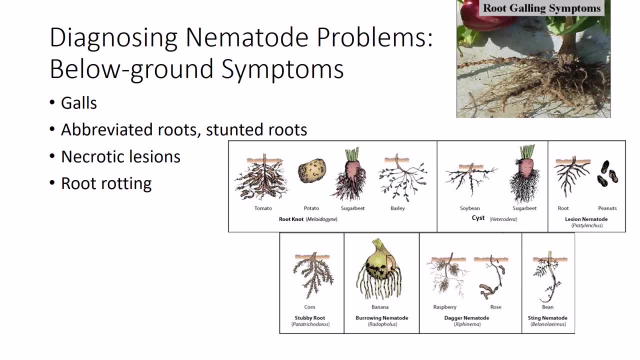 on roots by root–knot nematode abnormalities, abbreviated roots or stunted root growth, necrotic lesions in the root cortex and root rotting may all be a symptom of nematode problem. An experienced observer can see cysts on the roots of their host without magnification. 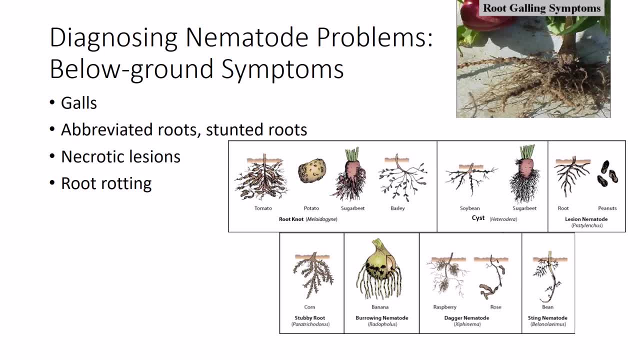 The young adult females are visible as tiny white beads about the size of a period on a page. After a female sits to the side when I call it–well when I get home they deeply get occurred. nematode dies. her white body wall is tanned to a tough brown capsule containing several hundred. 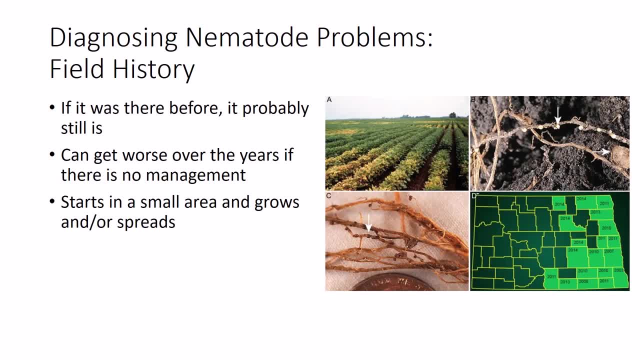 eggs. Accurate field history can provide valuable clues to the identity of nematode and other pest problems. A nematode that has been present in the field in recent years is probably still there and is likely to injure susceptible crops if environmental conditions are favorable. 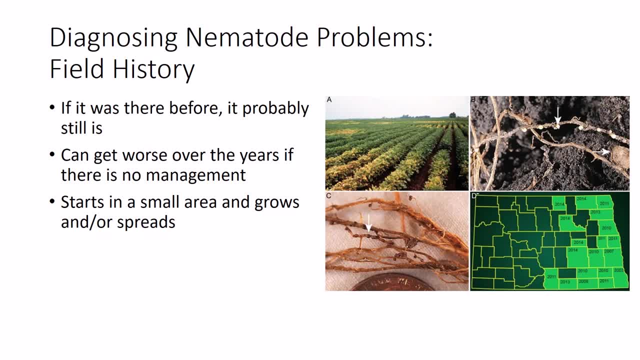 Production records that show a gradual decline in yields over a period of years, despite no change in cultural practices, may indicate progressive development of a nematode problem. A nematode infestation in a new field usually begins in a small area. It gradually intensifies. 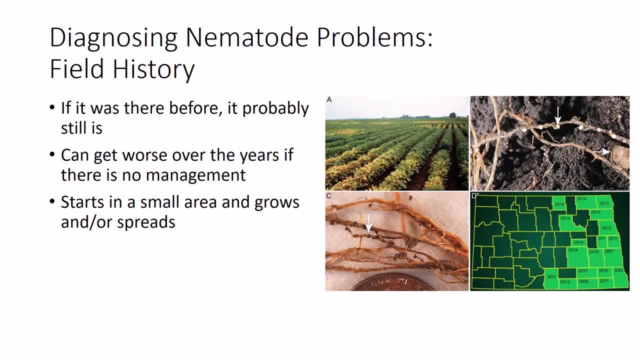 in the original spot and is spread through the field by cultivation, harvest erosion and other factors that spread infested soil or plant parts. Therefore, the total effect of a recently introduced nematode is a gradual production decline for the field as the